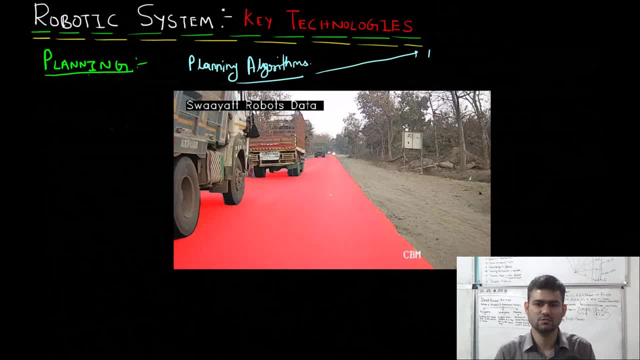 Sometimes we call them in the context of autonomous driving, we call this motion planning and decision making. Okay, So typically the planning problem for a robot is broken into three or four different pipelines. so these are pipelines of components. So these components are route planning, or sometimes we call it mission planning. 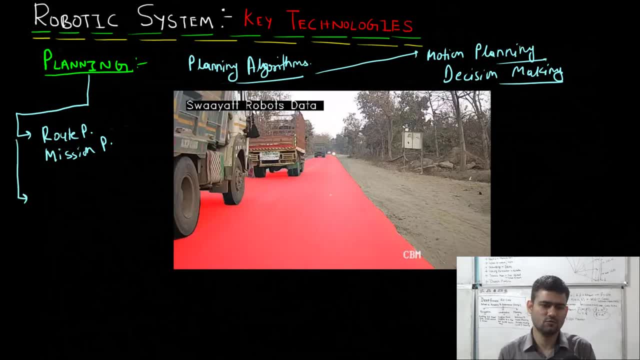 The next is trajectory planning. So trajectory planning is the process of planning a robot, So trajectory or a trajectory, or motion planning, motion planning, trajectory planning and also path planning. The third component is the behavior planning or the decision making algorithms. 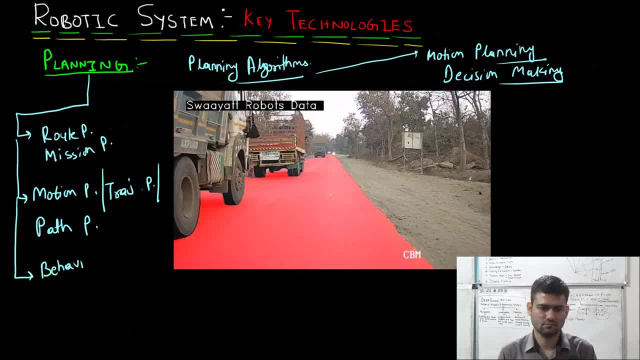 Okay, So three components are motion planning. The next component is the path planning. Okay, behavior planning or decision making algorithms. Once we have planned, so the decision makers and the motion planner or trajectory planner combinedly produce a local trajectory and a set of behaviors along the trajectory for 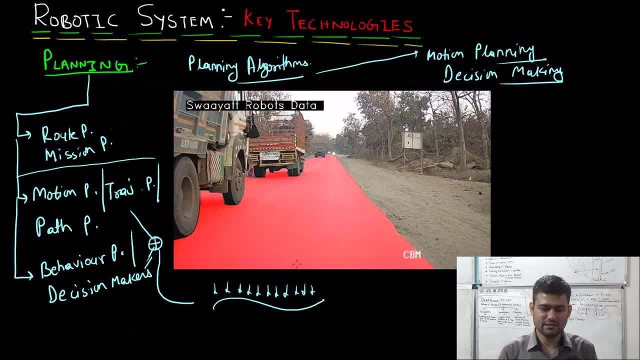 a robot or a vehicle to execute, And these behaviors and this trajectory is executed by a set of control algorithms. Okay, For example, in the context of autonomous driving, no matter what behavior plan or what trajectory plan you come up with, ultimately you will have to convert that plan into following. 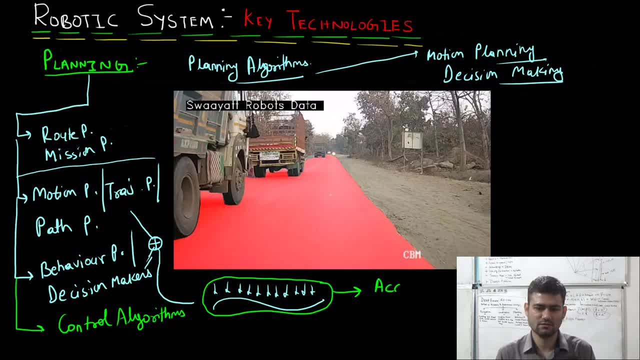 You have to sort of break it into the accelerator command, or perhaps if you are having a manual transmission vehicle, Then you have to also have a command for the clutch. Most importantly, you will have a command for brake and accelerator- sorry- and steering. 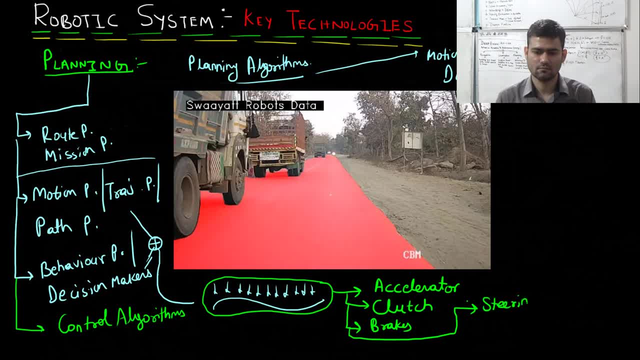 wheel. Similarly, let's suppose you are having an industrial or warehouse robot where the robot, instead of being an equipment, So the engines that the vehicle, so the vehicles that have a steering wheel are. they follow the Ackerman dynamics principle. Now let's assume that you have a differential drive robot, perhaps a two wheel or four wheel. 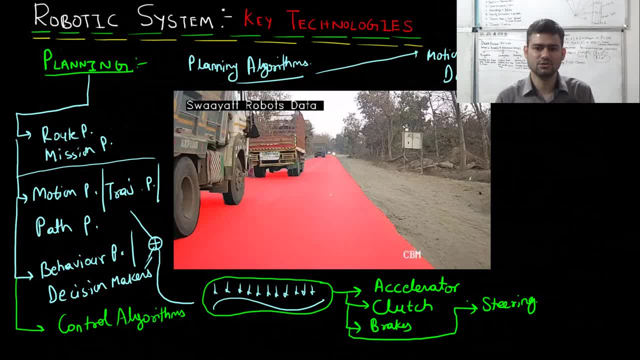 differential drive robot. So in differential drive robot, perhaps you would generate a command for the speed or the velocity of the left wheels And the right wheels. Okay, Okay, Okay, different velocity commands for the left wheel and the right wheels, the robot can. 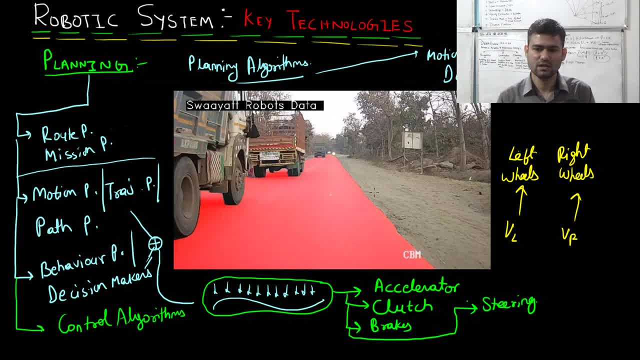 turn, move and go at a certain speed. so based on it, based on a robotic system, will have a different sort of control algorithms. so these control algorithms take the high dimensional plan as an input and they break it down into the low level control or motor commands in a robot or an autonomous vehicle. 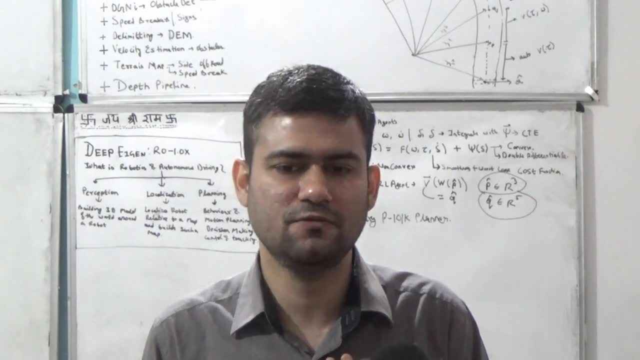 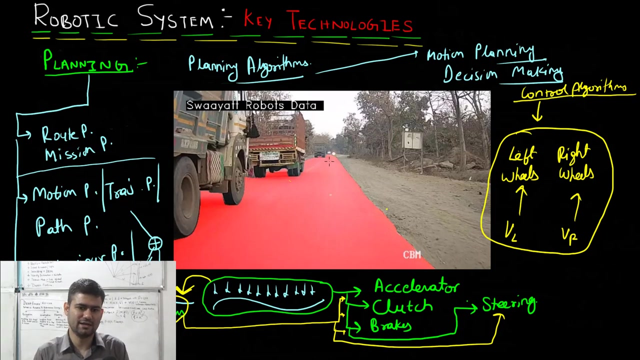 so, to give you a brief, high-level idea as to what planning in an autonomous train vehicle would look like, let's consider this image as an example. so, again, this image is captured using the cameras mounted on our autonomous train vehicle and, as you can see, like we have had an algorithm that detects where 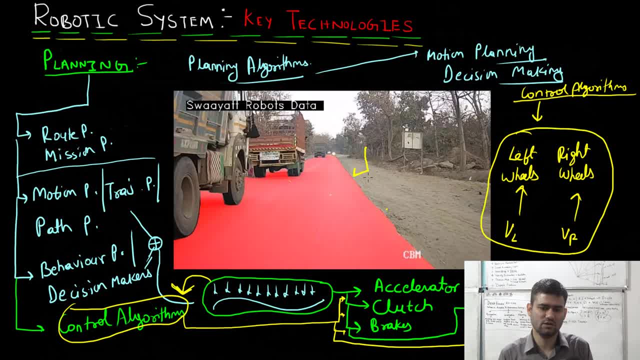 the road is. so, having understood the perception and and localization Gotham's, we know that the perception Gotham's compute all the necessary information for an autonomous vehicle, for it to build a 3d or projected 2d presentation of the world around it. similarly, we have seen that localization 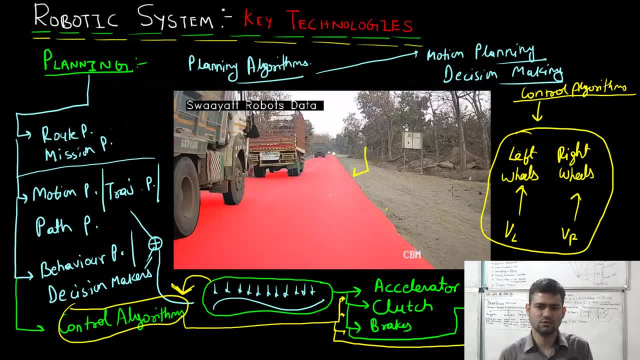 algorithms localize a vehicle on road so that it is it, so that knows where it is on planet earth and depending, for example, most of the autonomous vehicles in the autonomous companies in the world, they are building the technology that is highly dependent on the global, accurate positioning of the vehicle on road so for them to function. 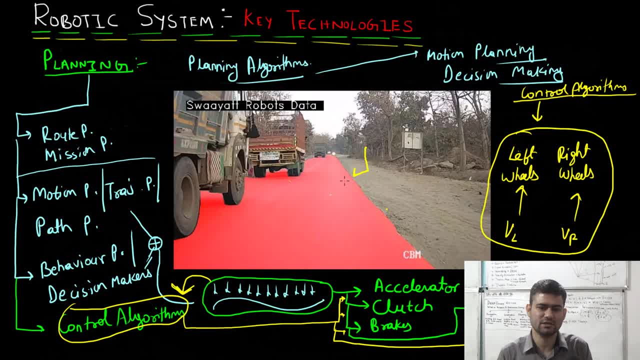 properly, they would perhaps require a 10 to 15 centimeter error in localization, whereas the technology that we are working on at soyacrobots we are not too centric on the global accurate position of the vehicle. but for the sake of the discussion, we don't go in the details as to what is important, what is not. important for down standing vehicle. lets consider the autonomous driving in general. now we have, let's assume that we have- difference between if you are using an artificial wheel or aston lights. fine, in general. now we have, let's assume that we have a very complex 55G control as compared to those that we have. what is supposed to be able to get better ride performance around for a vehicle. for example, saturn wicked runs well, it automatically goes to the join vehicle. we then have to, don't, don't? it's time to get good 1 time reasons. we need to be able to get the 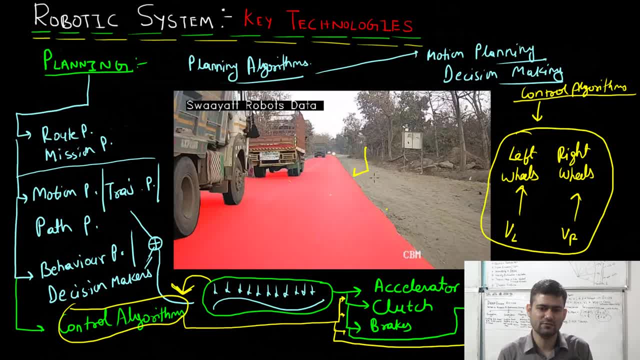 that we have again localization Gotham's that can localize a vehicle with perhaps 10 to 10 to 20 centimeter localization error. and let's assume that we started from point A and our goal is to reach a point B, so the route and mission planning problems. so let's suppose we have a road network. 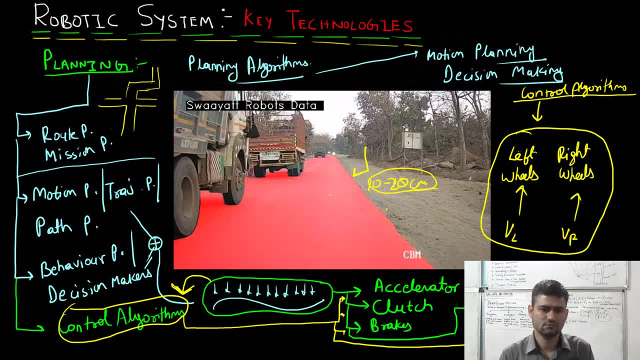 that looks something like this, and let's suppose our goal is to reach this point B and we started somewhere from point A. so a route planning algorithm or a mission planning algorithm will plan a global route for the vehicle to follow and and this route planning- whether the, the mission or the route plan- takes this approach or this. 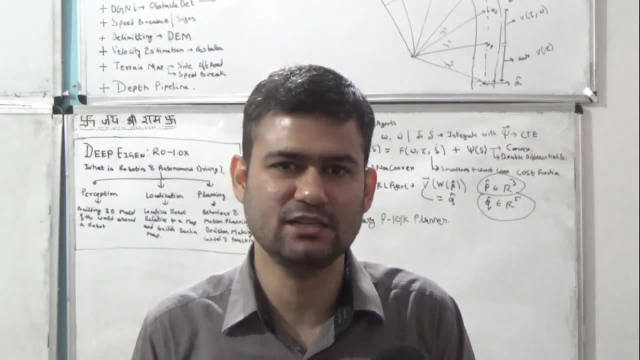 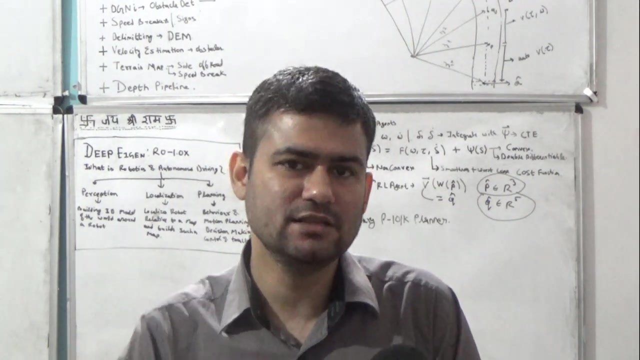 approach. it depends on various factors. for example, we can take the traffic into account. we can take the road tearing into account. we can take the uh. for example, we can have a cost function that uh heavily uh penalizes the length of the of of the trajectory, or the distance the vehicle. 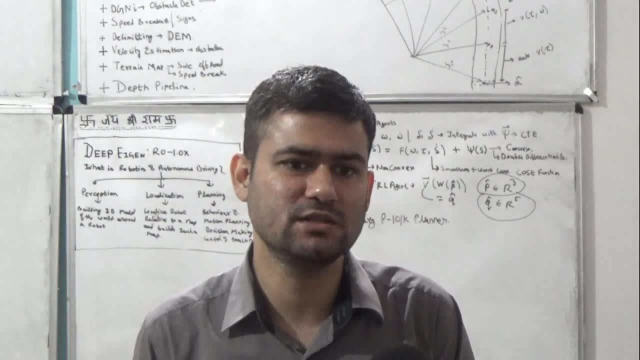 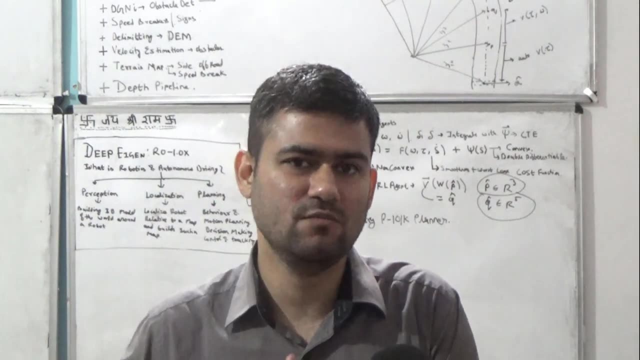 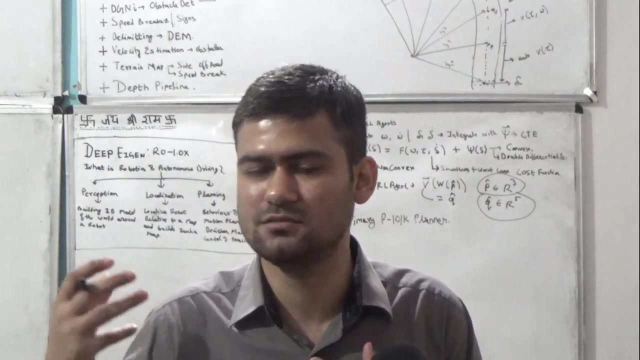 has to cover. so in that case, the mission or the route planner will select the path uh that is of minimum length. uh. likewise, we can penalize the time required to reach the destination. in that case uh, the route plan or the mission planner will take the the traffic scenario into account. it can take several other factors into account. it can take: 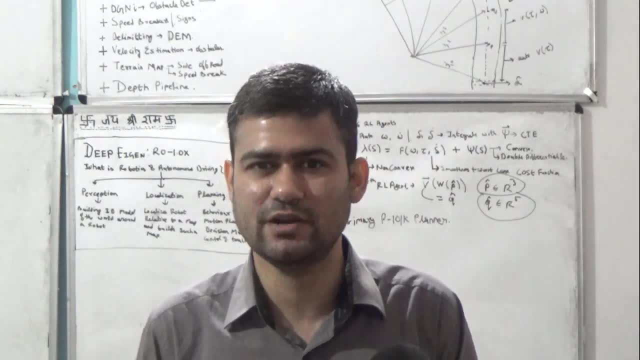 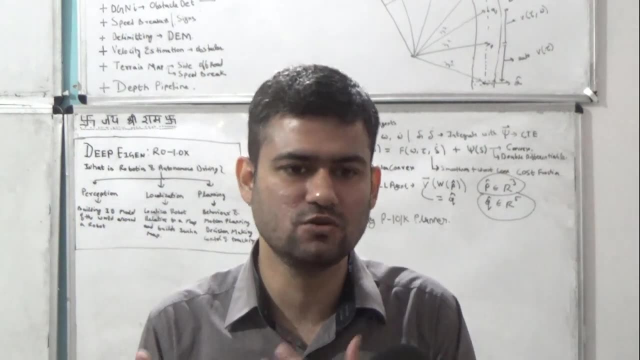 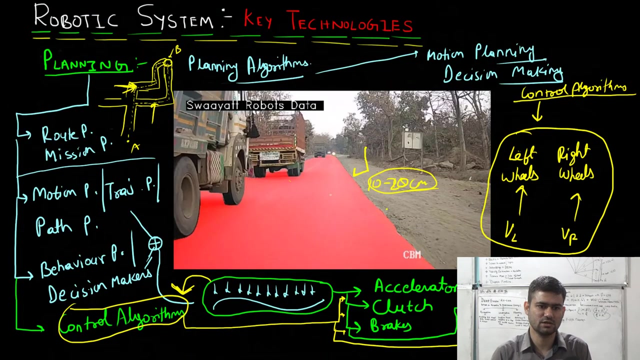 the terrain map into account. because the terrain is rough, then the vehicle would navigate its slow speed. the training terrain is smooth, then the vehicle can navigate very high speeds. so, taking the various factors into account, the route or the mission planner uh will come up with a global plan for the vehicle to follow. let's suppose it it selects this route. 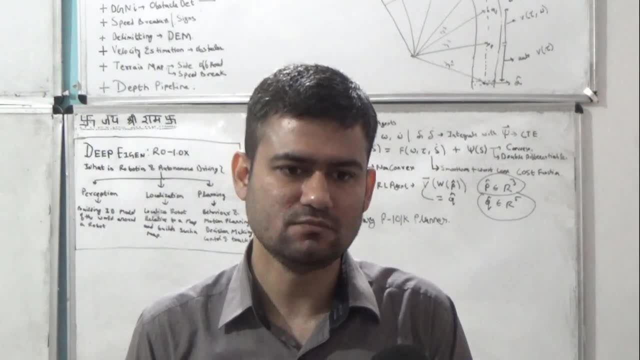 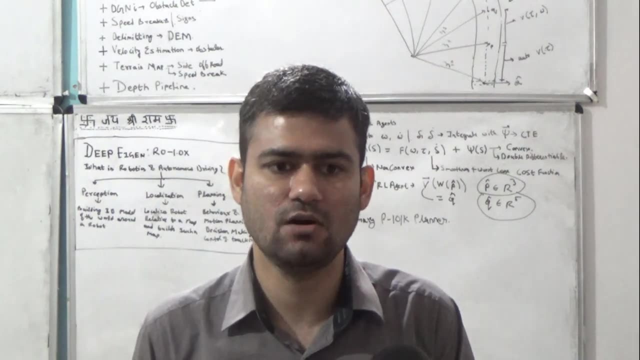 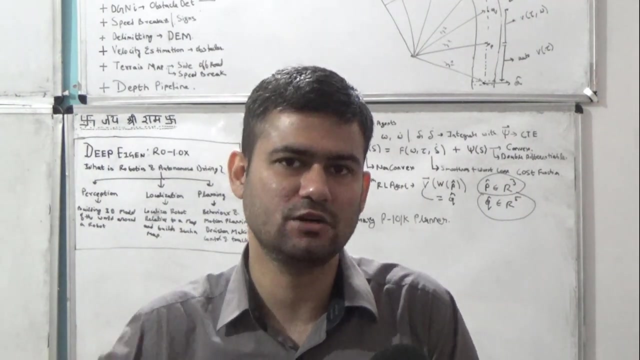 so once the vehicle knows where to go um, then it's all up to the perception and the planning algorithms for uh to take the vehicle safely to its destination. localization again, i mean uh. some companies depend heavily on global accurate positioning, but we, on the other hand, at swyatt, are developing uh cutting edge. 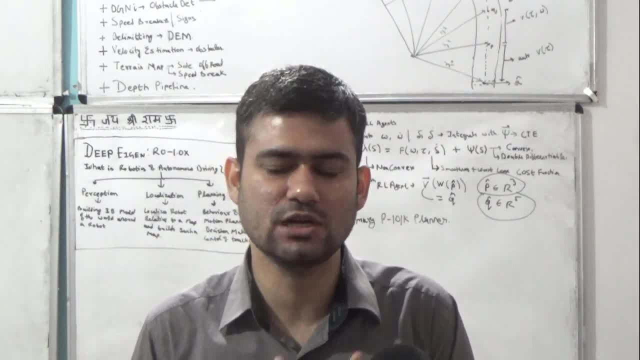 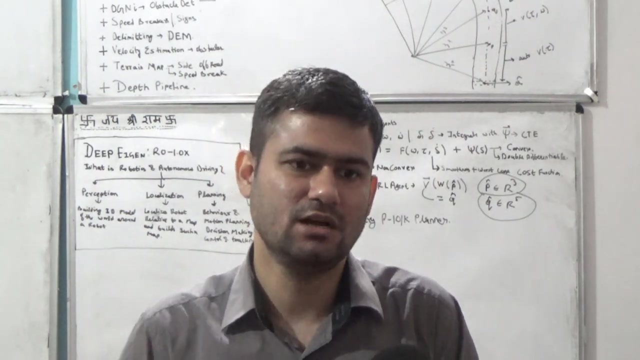 technology? uh, that doesn't require global accurate positioning of the vehicle on road. it just uses local relative localization for uh for for keeping the vehicle safe on road. but uh, keeping that discussion aside, let's assume we also have a localization costums that can uh localize a vehicle on road with 10 to 20 centimeter. uh, you know, error in localization. so in that case, 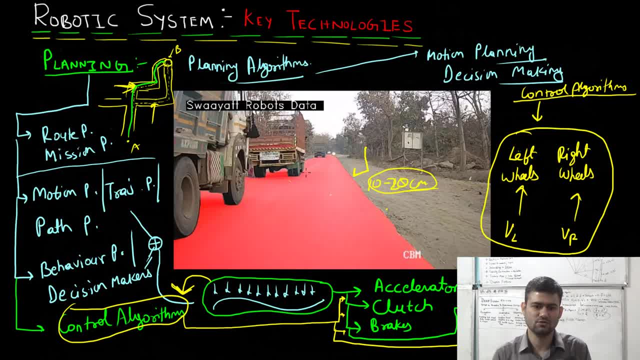 um, let's assume that the vehicle is navigating on on this road, right? so what are all the uh algorithms that this vehicle would need to actually, uh, you know, execute all its uh many words safely to reach the destination? perhaps, uh, the one first, the very first algorithm: we 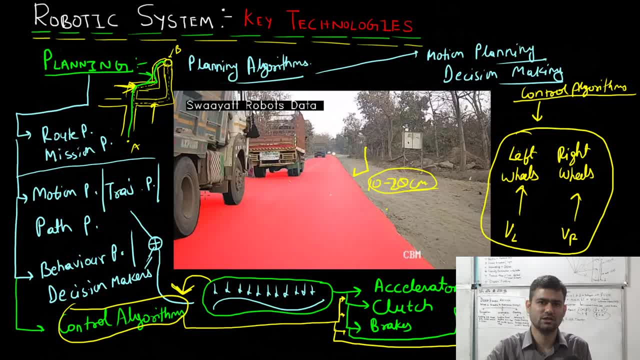 would need is a route planner. the route planner is already give has given us a global trajectory for the vehicle or robot to follow. so, assuming, uh that, that the route planner, or a mission planner, has already provided us a road network to follow, um, it wouldt only want to narrow the radius of the route planner top shown here. 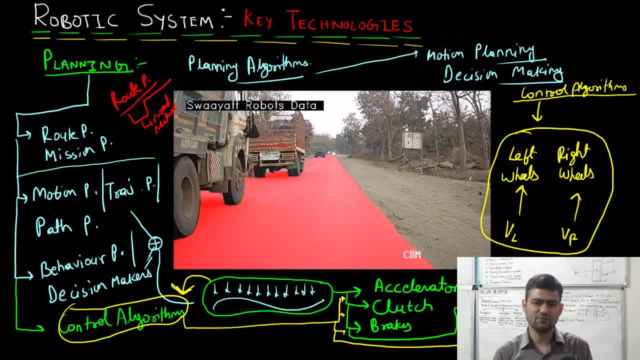 up here. down below is the route plan to the discussion about how it can be handled by the range of four 빵f ribosances that are there. now its us hog agu, okay, so now lets g dysfunction elected and open, and so we know this is the objective of the spring. price. that is something which you canientos and lots of things that we have to make sure to accept: driverias where we know all the turns and exists to take to reach our destination, and assuming that we have the perception algorithms that can detect all the necessary information, for example, road, perhaps, lane markers and road boundaries- uh, perhaps you have algorithms to to to build a terrain map- assuming that we also have algorithms that can compute the velocities of the obstacles on road and all any any necessary algorithms that we need to compare and to go to them is traditional for various purposes. 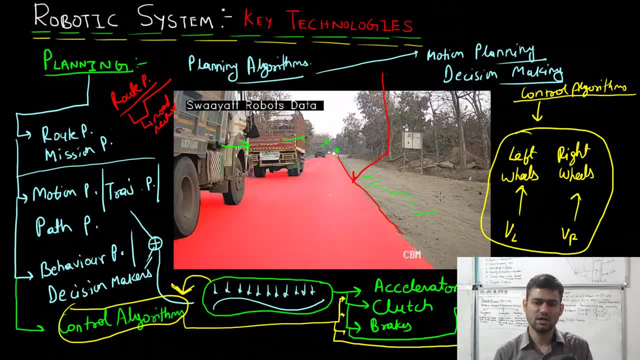 need to actually perceive the environment. assuming that we have all such algorithms, and assuming that we also have localization algorithms, that can, you know, position the vehicle accurately globally with 10 to 20 centimeter precision on road. so to so consider this image as an example, let's suppose our vehicle is navigating on this road. 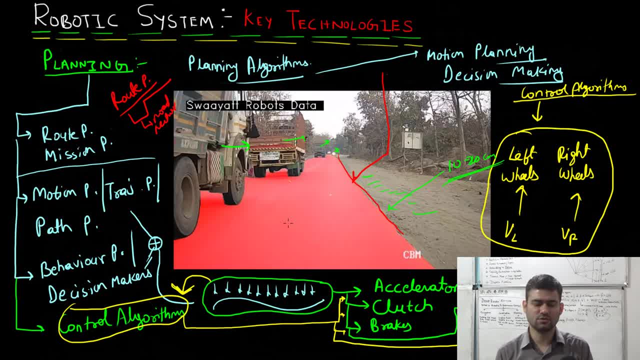 so what are all the algorithms, what are all the planning algorithms that would be needing to keep the vehicle safe on this road, as well as enable the vehicle to reach its destination? so perhaps the very first algorithm we would be needing is a local- uh, you know- trajectory. 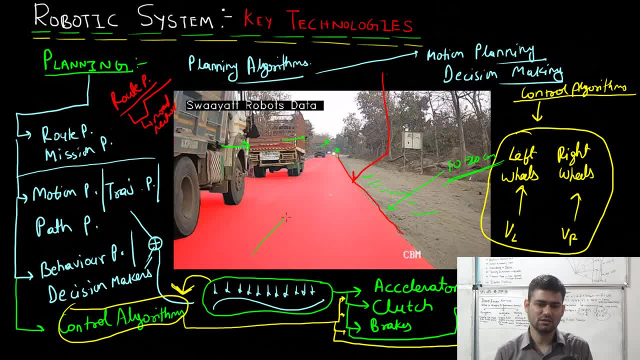 planner or a motion plan or a path planner that plans the trajectory of the vehicle. let's suppose it looks something like this: uh, then we would be. we can see that. uh, since this is a generalized electronic vehicle, and assume, when you are driving a vehicle on road, what are? 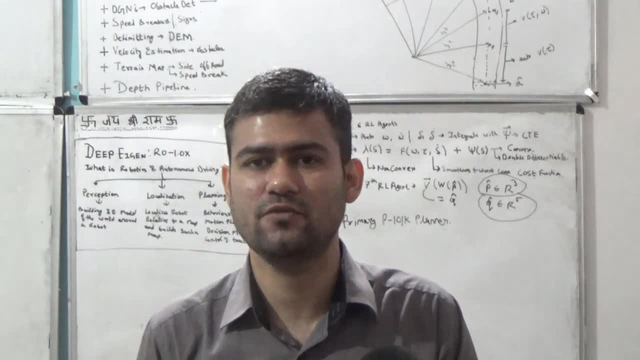 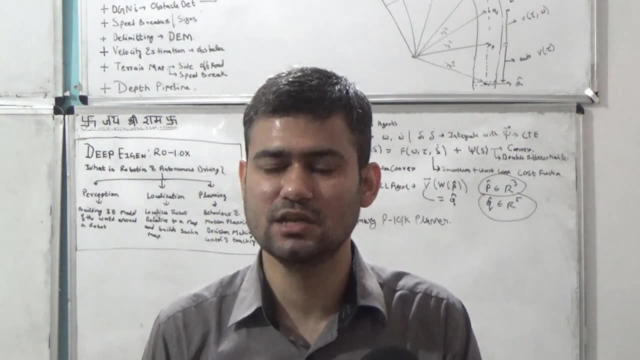 all the decisions that you make when you're driving a vehicle. you make decisions like what a speed to uh to drive at you you. you make decisions about overtaking other other vehicles if you're already in the midst of overtaking- and, as you know, in india i mean on typical two lane roads- when 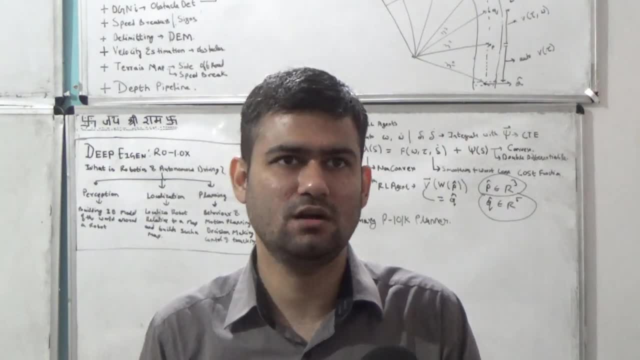 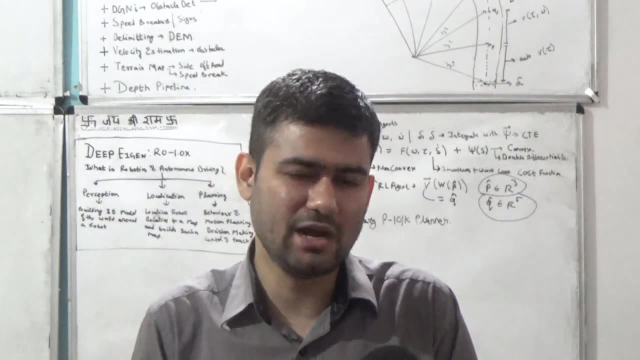 there's a traffic coming from the other direction, you sometimes, uh, you know- make a decision to about your overtaking. if you feel that this overtaking is not going to be successful, then you're about, so perhaps you may need a decision maker for that, uh, perhaps- uh, i mean again if you're driving- 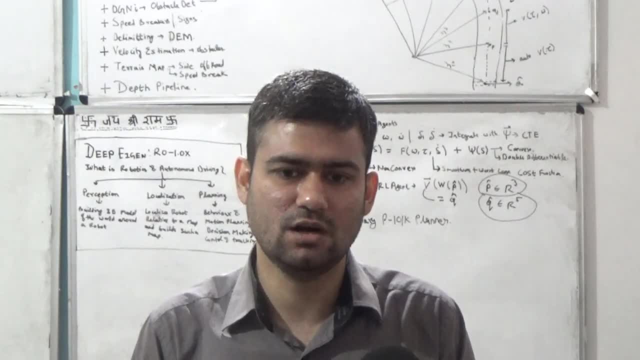 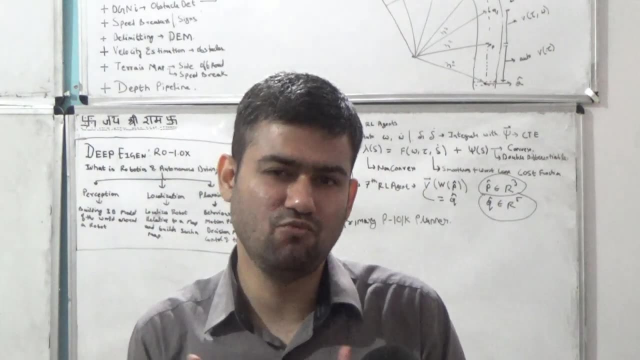 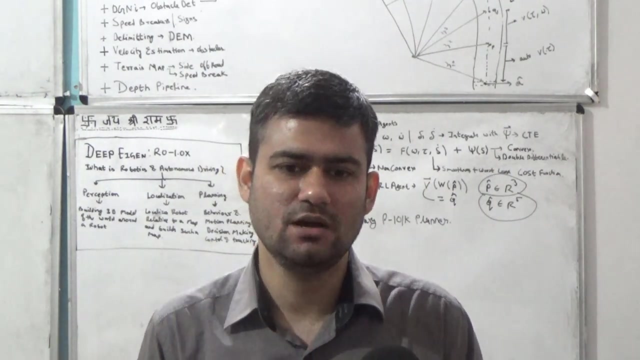 in india, you know that sometimes you have to yield away to a truck or or other vehicles coming from the other direction, so we need to have a decision maker that decides when to yield, how much to yield, at what speed to yield right, because it's a multi-agent game that we're playing on road. 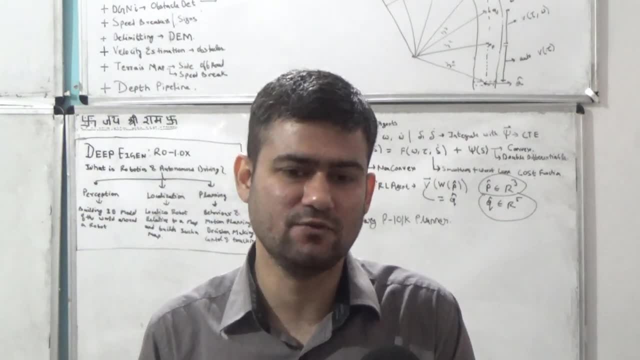 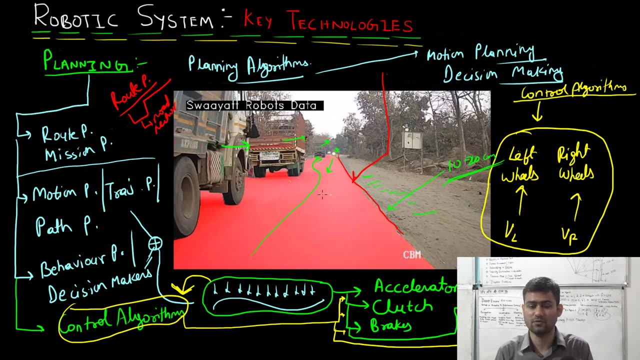 right, so we'd be needing, perhaps, all social gods to actually keep the vehicle safe on road. so, uh, perhaps you would be needing, uh, for example, to to conserve, for example, the problem of voting vehicle is currently in the midst of overtaking, so we are overtaking this, uh, these trucks, and we 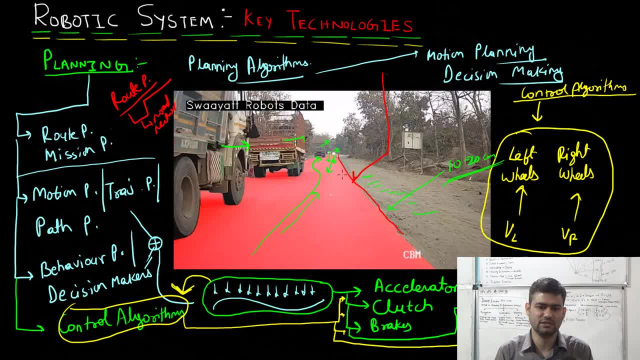 can see that there is a car and a bike that is coming from the other direction. so perhaps we need a decision maker that takes the velocities into account, that takes the dynamics of the ego vehicle into account, it takes the dynamics of the other obstacles into that, takes the dynamics of the other obstacles in the other vehicle and then, if we can take the 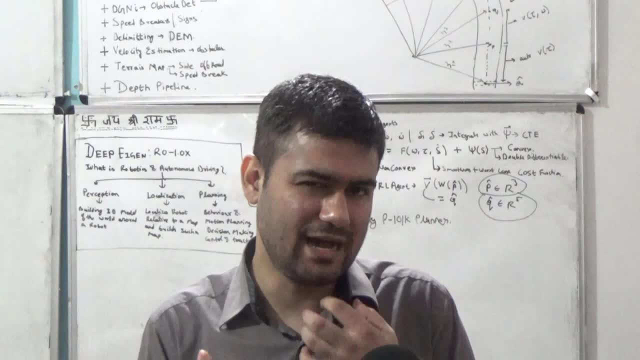 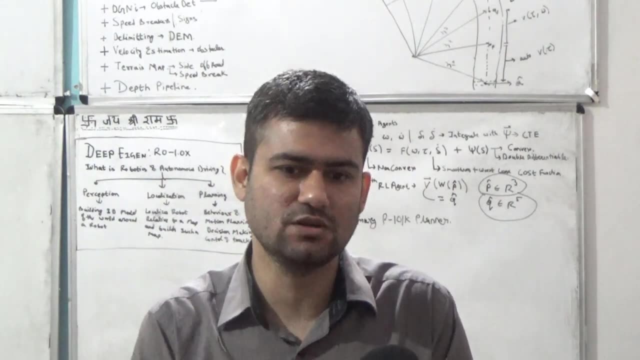 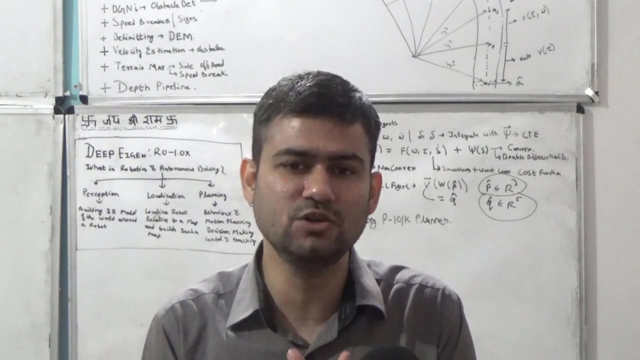 account and taking all the factors as to what actions we can execute and what actions other obstacles or the vehicles in the environment can execute. let's suppose this algorithm has a capability to do value, to take all this information and and and compute the probability of a vehicle being safe and based on that, 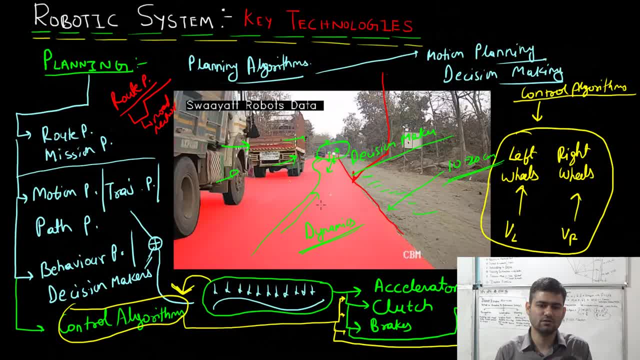 probability, it decides whether to keep on this overtaking or to abort the overtaking right. similarly, we would have an algorithm that initiated this overtaking, and likewise, we would have an algorithm that perhaps decides whether the overtaking first, first, should end with this truck or they should keep on. 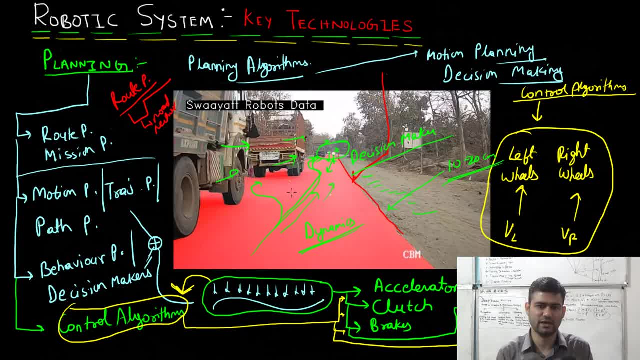 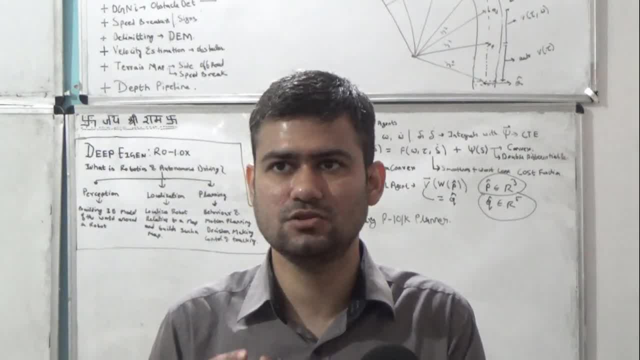 continuing with two trucks in a continuous fashion. right, so you can see. I mean the number of planning algorithms or the kind of planning algorithms that we're needing to keep the vehicle safe on road. it again depends on application. for example, if you are driving in an industry, 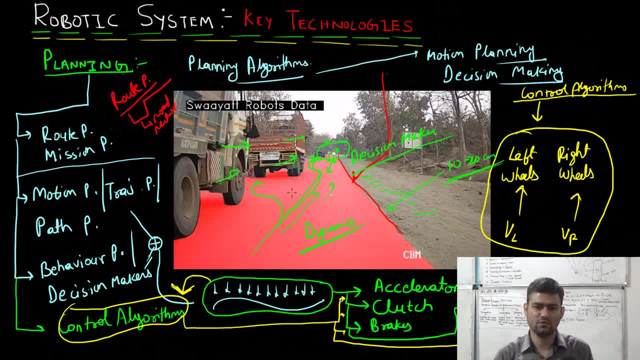 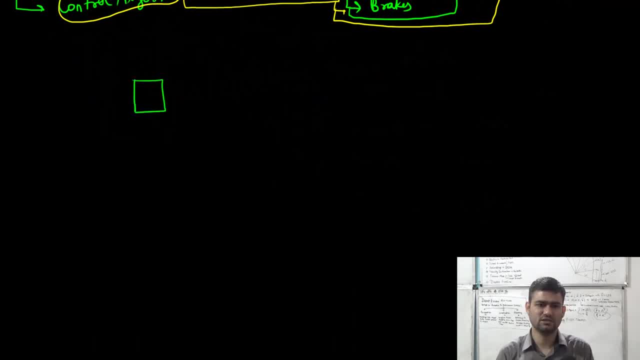 setting right. let's suppose you have a robot that is driving an industrial setting and let's assume that they are very narrow roads, so assume this is a forklift, this is an automated forklift and this is the forklift review for the forklift. 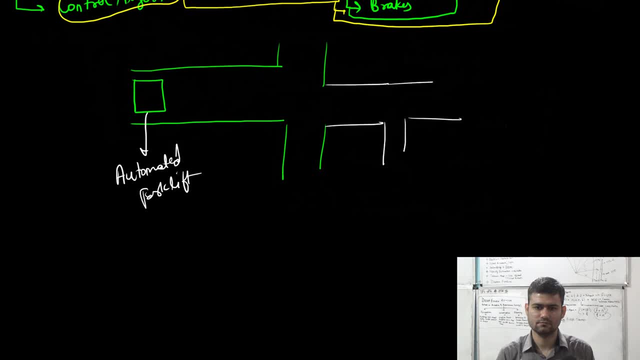 as each one is moving out of the Veily forming, and this is my typical Kashmir. instead of mail in a different сер48, and if I turn off my per Epic until six, that would inform me right here. this Forklift is navigating at perhaps a many minutes per hour or two minutes as an customers. more depends on Apple personalALLY. utiomail on this Factory got certain characteristics and these are some of the blind spots. so these curve line supply 2ound. these are blind spots and it is drivinganger shopping in this industrial corridor and these are, you know, some of the blind spots. so these are blind spots and it is driving in this End meta and I assume that this forklift is navigating. I guess that this forklift is also. город can't solve this starts. 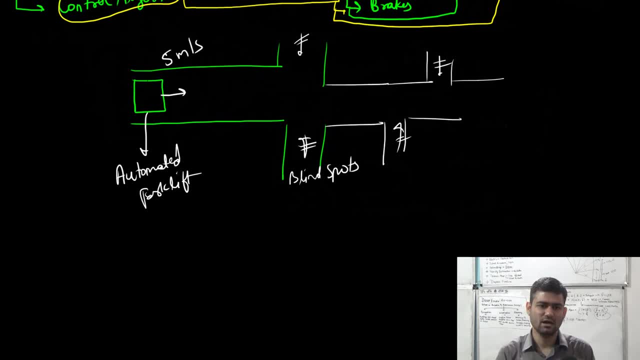 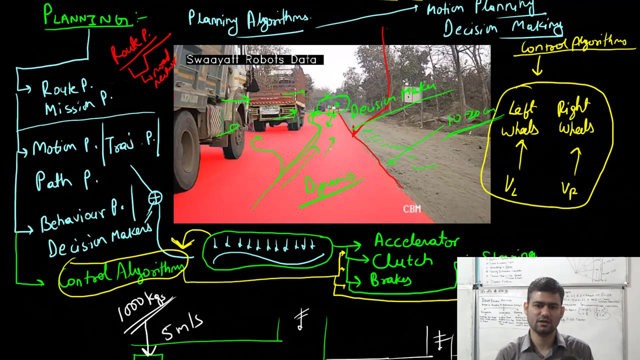 uh, maybe five meters per second and is carrying a load of thousand kgs. so in case of an autonomous vehicle, let's suppose, uh, if we have the traffic coming from the other direction and the decision maker decides to slow down, so perhaps we would have a decision maker that decides whether to slow down. 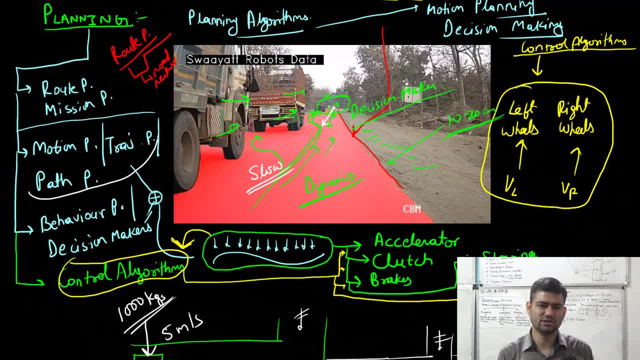 or not so? motion planner, the, the algorithms that plan trajectory, they can inherently compute all these. you know the speed that the vehicle should be, uh, should be navigating at, based on the speed of the other obstacles and the and the vehicles on road. but additionally, we have too many decision. 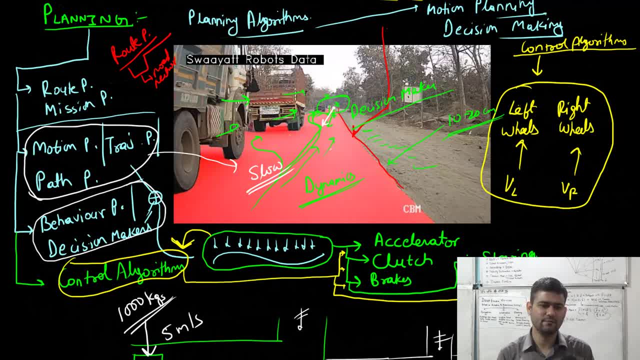 makers as well in our transferring vehicle and they work in parallel to to keep the vehicle safe on road. so there's a. if we are talking about a generalized drawing, then there's a lot of information sharing. that happens between a trajectory planner and a decision maker, so so there are too. 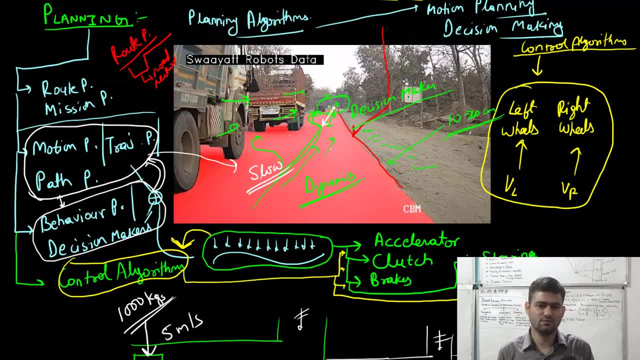 many decision maker, for example in software's autonomous running vehicle. uh, in typical experiments that we do on tight roads, there are roughly 15 decision makers and there are roughly three different motion planners that plan the motion of the vehicle on the road, coming up with the, with the with the time parametrized trajectory. 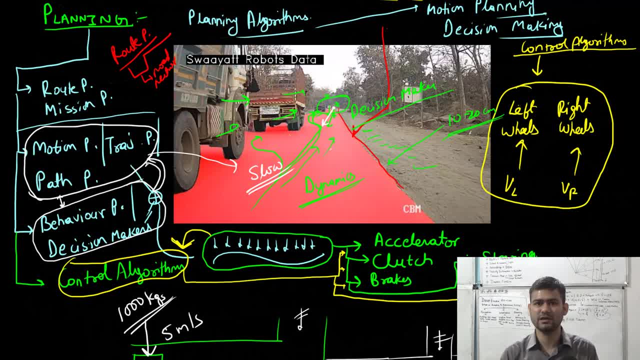 uh, whose task is to keep the vehicle on safe. additionally, we have decision makers that are also trying to keep the vehicle on safe, so they work in parallel and there's a lot of for information sharing, and typically the behavior planner appends the decision on the trajectory that is computed by a motion planner, and this is 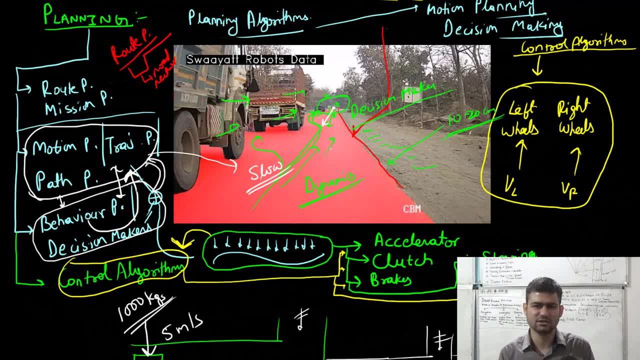 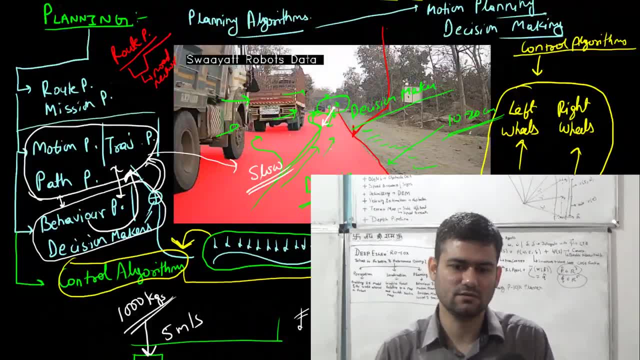 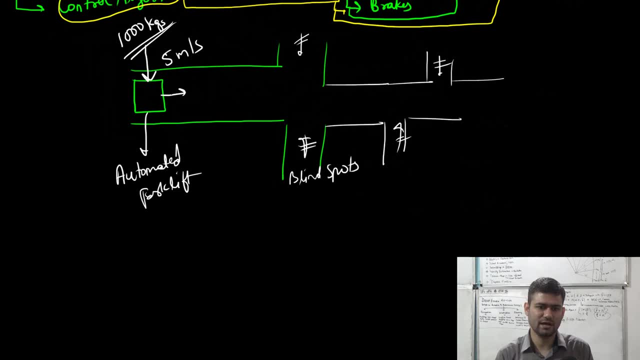 how an autonomous vehicle works. it's a very complicated, you know, discussion, but we will just like restrict our discussion to give you a very high level idea as to what planning algorithms do. we'll just restrict our discussion to this industrial robotic scenario. so assume that we have a robot that is. 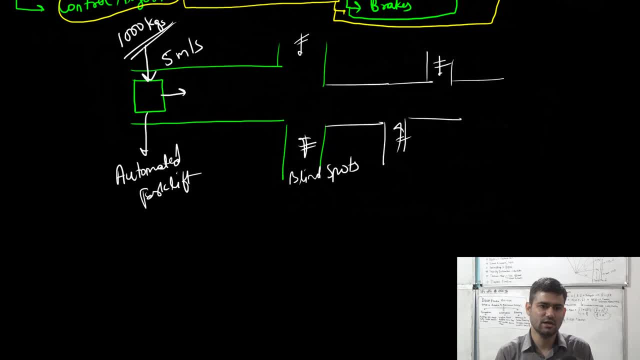 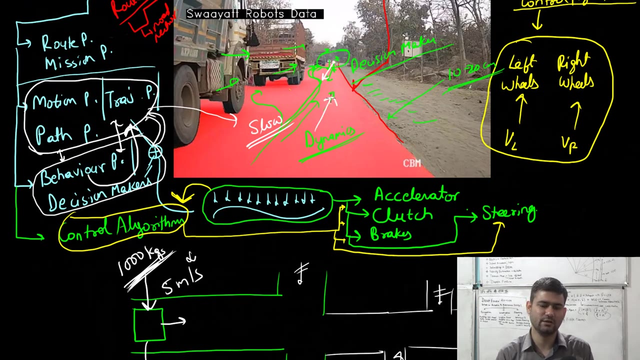 navigating an automated forklift navigating the corridor carrying a thousand kg weight at five meters per second. so an autonomous vehicle. if it needs to slow down, it can apply the brakes. for example, if we are feeling and that there's going to be an imminent collision, we can apply hard breaks at. 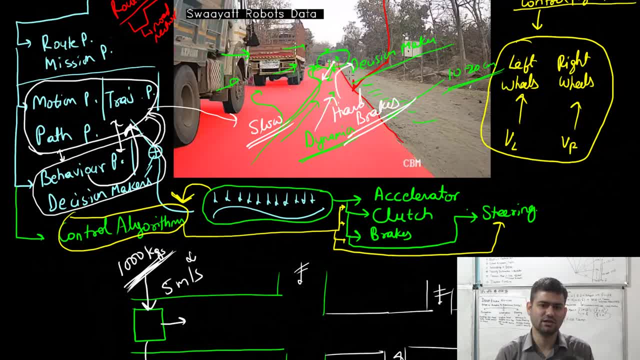 the same time, we can apply the steering command as well to actually steer away from that collision if the vehicle is not being able to steer and that collision will happen and the vehicle is not already in what we call inevitable collision states. we would be discussing all these concepts later on in module 4 as to what typical path planning and 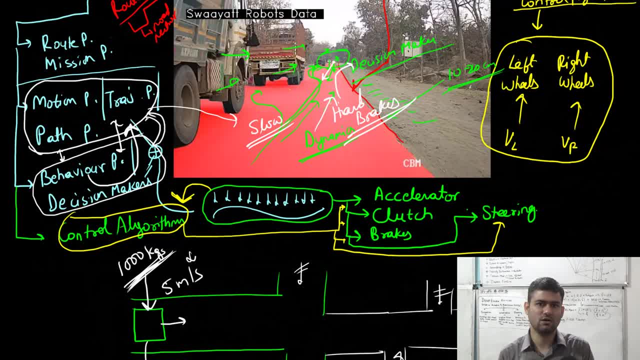 motion planning algorithms there are, what the dynamics of a robotic system and what is an ics inevitable collision state. so we'll be discussing all these concepts in the module 4 of this course. so we don't care as to what these algorithms or what these terms mean at the moment, we are just just discussing. 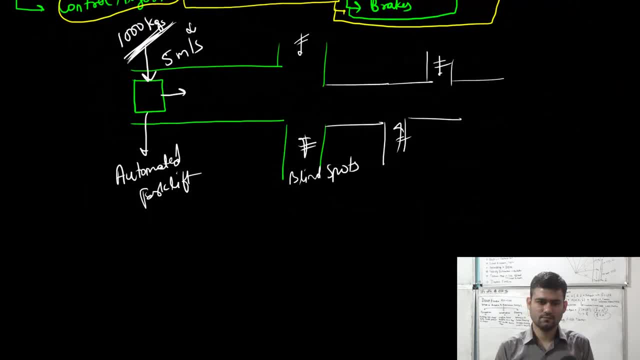 the field at large. so in case of this forklift an autonomous vehicle can apply hard brakes. but if we apply hard brakes in this forklift at five meters per second, at thousand kg load, then there's a chance that this entire forklift may just topple right. and we will be discussing all these concepts. 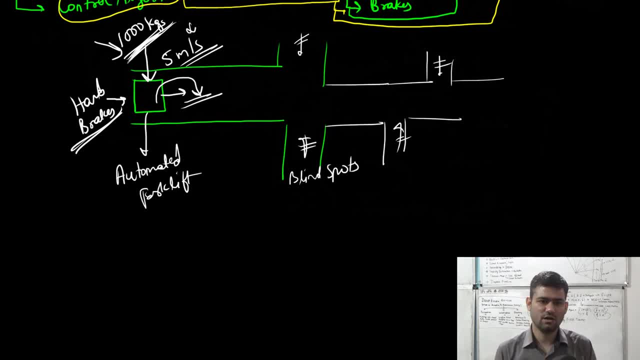 그대로. take at leastっ 10% of a situation- Diego cable situations, for example. if a person certainly comes in front of this forklift from this blindings spot, then this vehicle, this Walkthrough, should have planning at Gotham's that take this uncertainty of a person coming from. 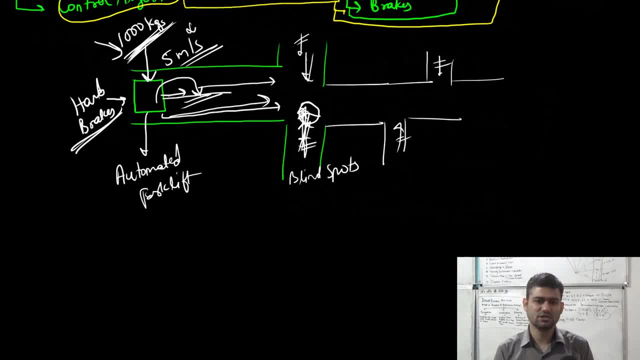 these blinded sports into account and select a velocity profile and trajectory at every given time. step that, even if such a situation happens, the vehicle shouldn't be in a situation that needs to apply the hard brakes which may result in toppling of this forklift, resulting in a huge damage. right so, in autonomous driving perhaps. 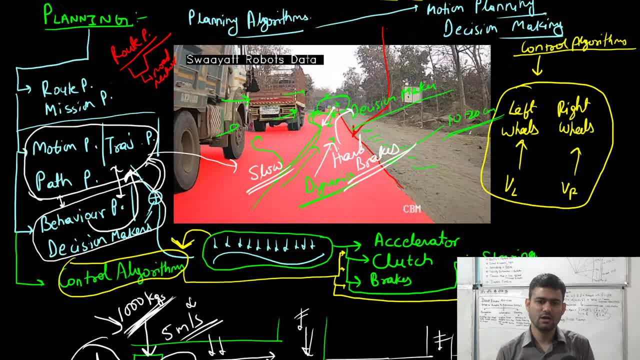 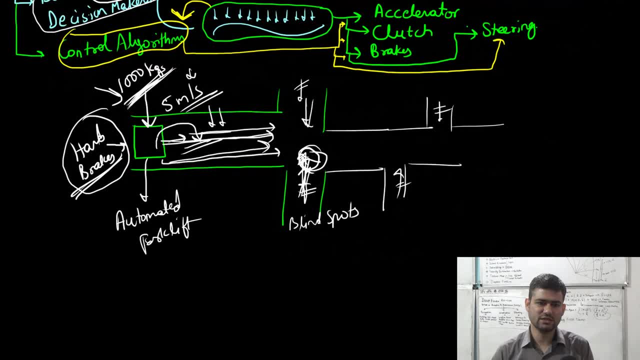 although autonomous driving is a much more complicated problem. but still, I mean we can apply hard brakes over here. just for example, in some cases we can apply hard brakes, but in an industrial setting with a thousand kg load carrying forklift, this may not be a good scenario. I mean to apply the brakes. so you see, 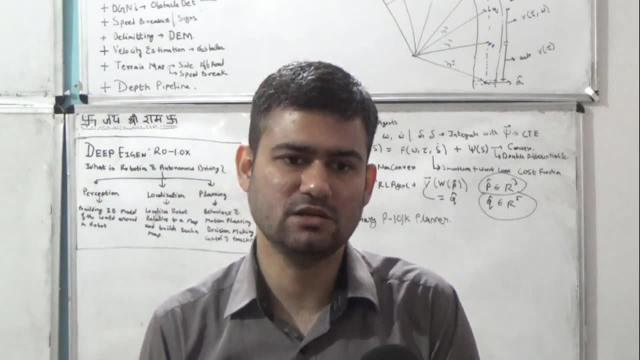 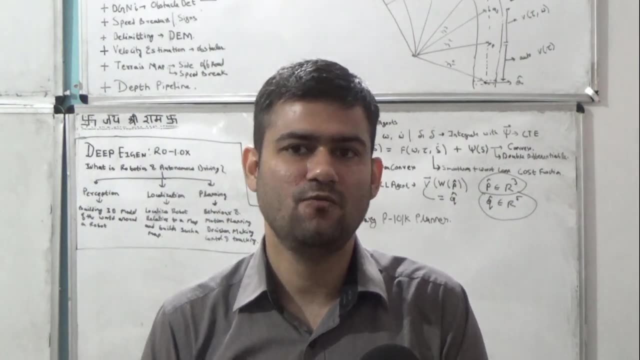 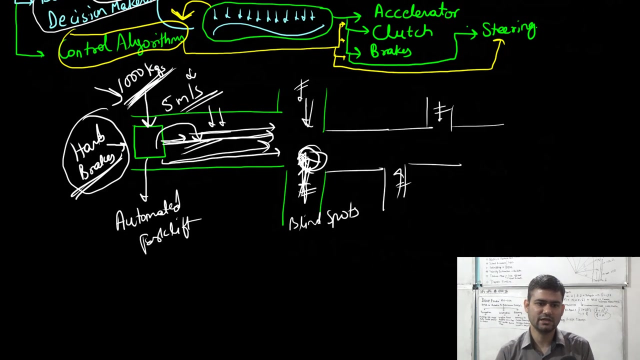 the kind of behavior planner or the trajectory plan of the motion plans that we're needing for this industrial robot significantly differ from the kind of algorithms that would be needing for an autonomous driving vehicle. furthermore, the localization of the robot in an industrial setting. the localization of the robot in an industrial setting. 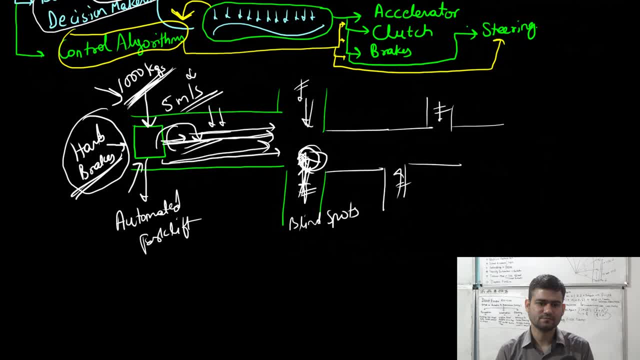 plays very important role. for example, you are carrying a load and the task is to place this load at a particular configuration, at a particular angle and a very specific position and a very, you know, particular orientation. so to execute the task of placing this load at a very specific position, with a very 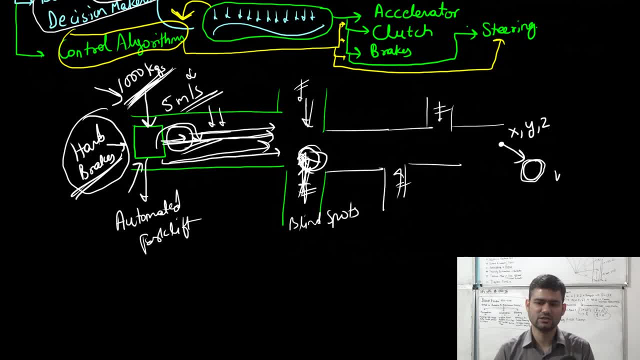 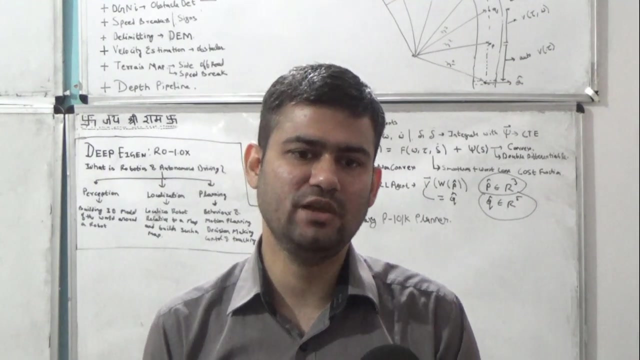 specific orientation, the margin of error is very small. localizing this forklift, related to the environment, is very important, so perhaps in this case we would be needing a localization error of 5 centimeter, or sometimes even less than 500, perhaps 2 centimeter localization error, right? so depending on the application of we. 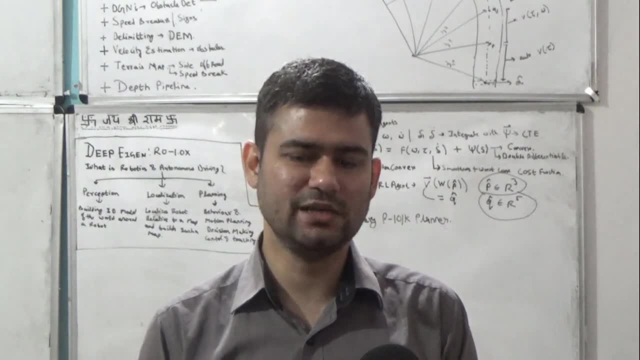 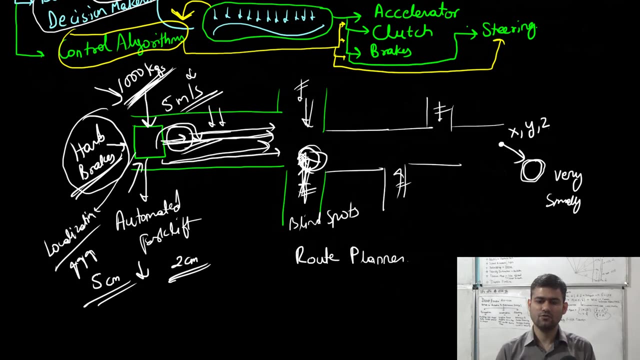 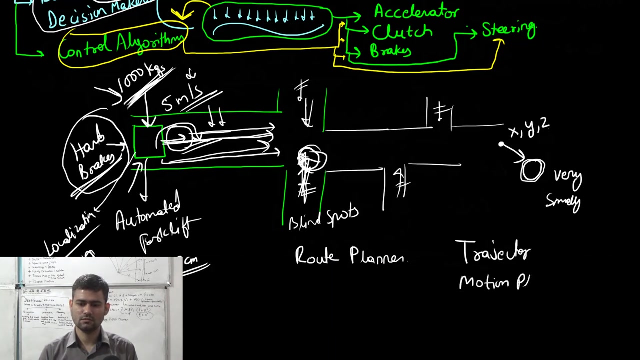 have different kinds of planning algorithms, but one thing is sure: that we would always be needing a route planner, we would be needing trajectory or motion planner. so we'll be using that- the term trajectory plan, or path planner or motion planner, interchangeably, although path planning. but eventually you're right that countries which 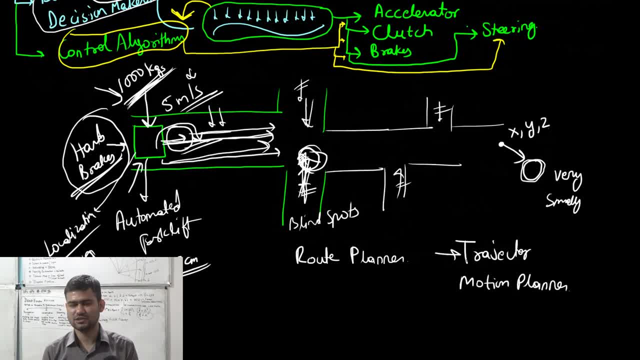 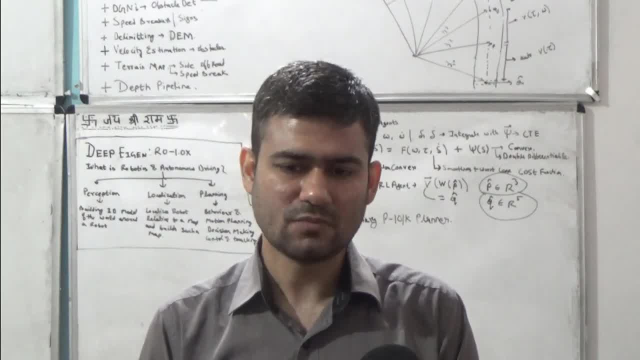 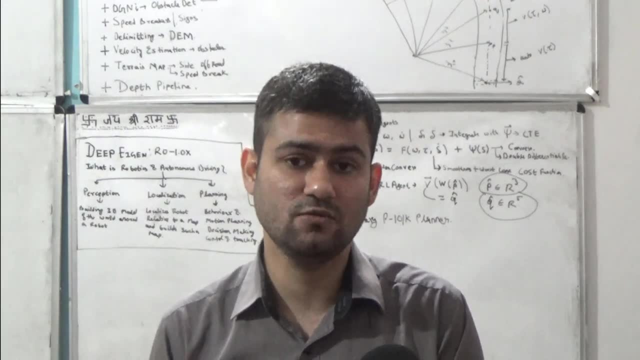 slightly differs from the motion planning and trajectory planning can be considered as a subset of the generalized motion planning. but we just use the these terms interchangeably and we would clear the differences between them whenever it is required or, for example, mostly in module 4 of this. 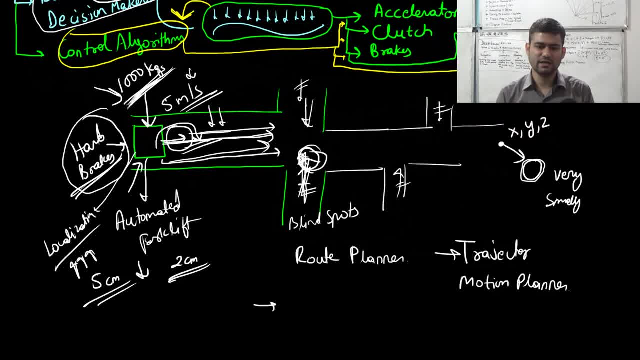 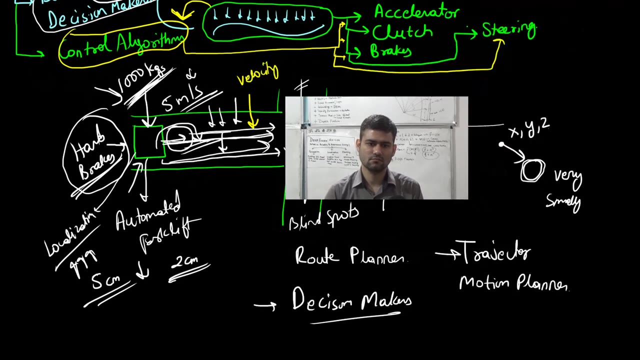 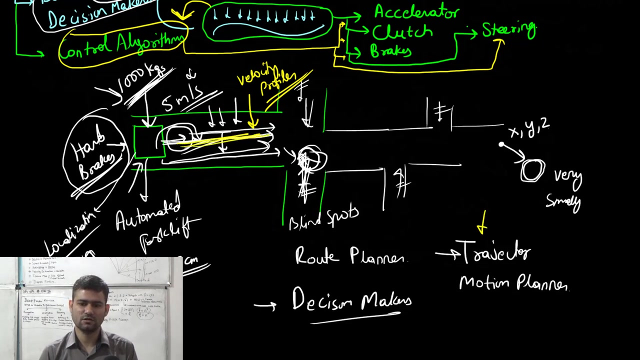 course, and what the other component that we need is, but is a set of decision makers. so decision makers take the future uncertain. It is into account and they, you know, have a lot of control over the velocity profile moments where typically a motion planner or a trajectory planner plan. so typically, 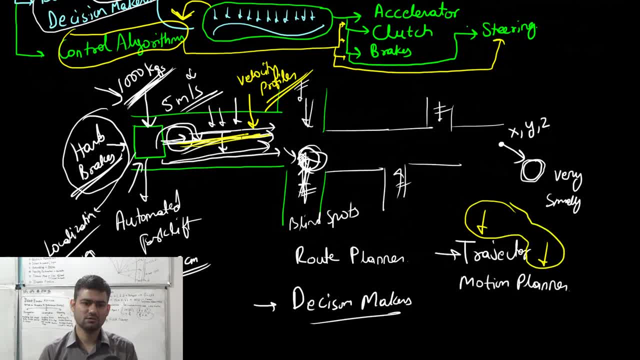 motion plannerasa trajectory planner output the velocity profile as well, but usually in robotics or in autonomous driving we don't follow directly the velocities computed by motion planner, even when we are doing what we call time optimal motion planning. In the time optimal motion planning, the motion planner would be outputting a trajectory that has x, y and perhaps z component, and it would have vx, the x velocity, the vy and vz velocity components that the robot should follow at each of the points on the trajectory. 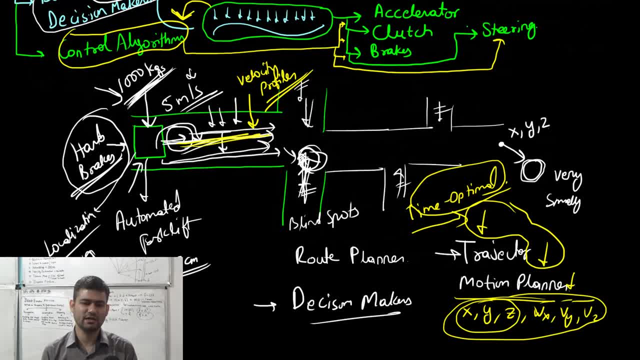 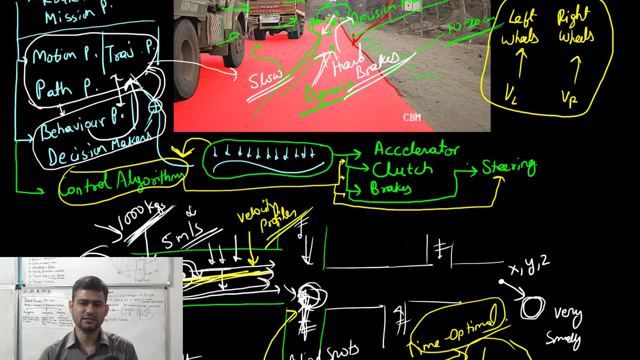 But typically it may be very hard to follow because typically the dynamics of the vehicles are too complex and we don't know how to follow them. We do not take the full dynamics into account while planning the trajectory And that is why we have a set of decision makers that control this velocity profile, that alter this velocity profile so that the vehicle can remain safe in an environment, taking all the future uncertainties into account. 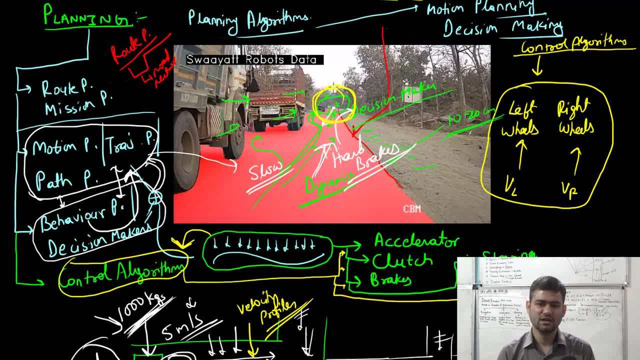 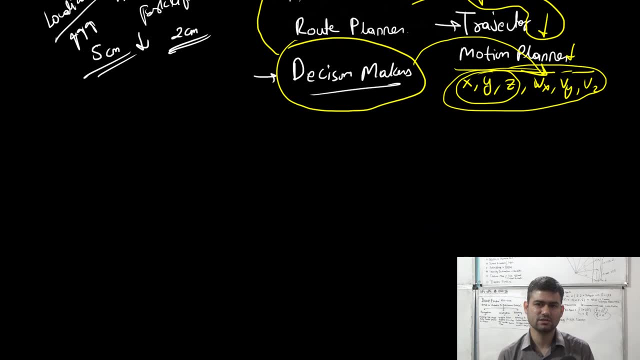 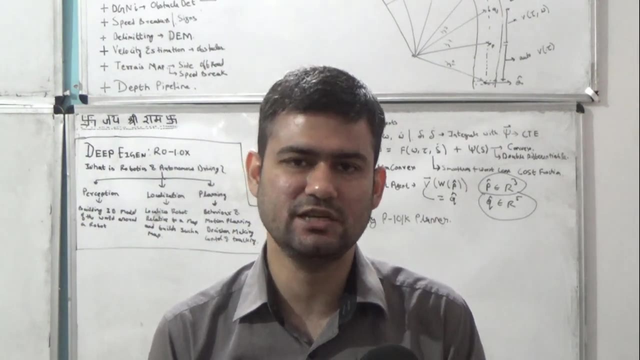 For example, these agents may change their speed and a motion planner may have a hard time in keeping the speed. They may even have to put a three wheel drive to keep the vehicle safe without having very specific decision making algorithms. And typically there is no end to the mathematics that you can read to make yourself a very good researcher or a very good engineer in planning algorithms. 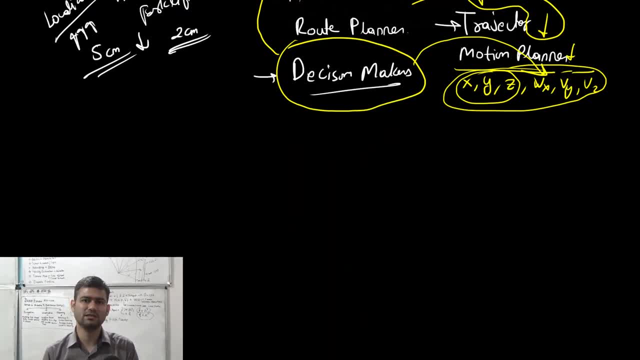 But typically in motion planning we use any field of mathematics imaginable to come up with a novel motion planning algorithm. also, there is no end to the mathematics that we can study to come up with. you know very robust decision-makers, but typically I mean to give you at a broad 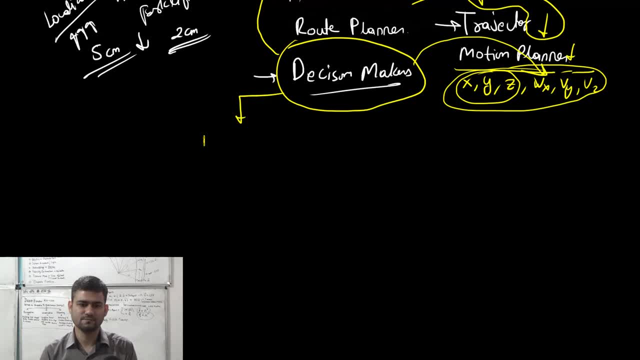 area. for example, if you are starting the field of decision-making, perhaps you can read a machine learning. you can study reinforcement learning. sorry, we can study game theory. we can also study mathematical or generalized like topological theory. we are using this theory heavily in motion planning at.